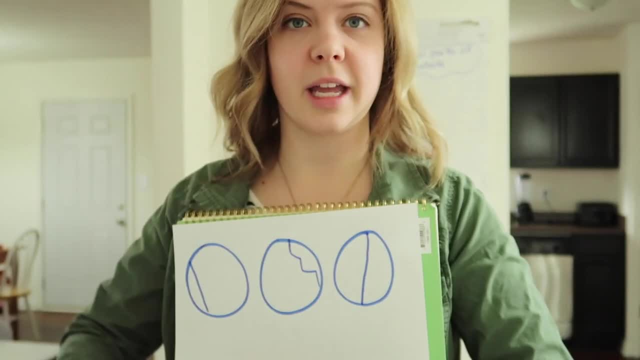 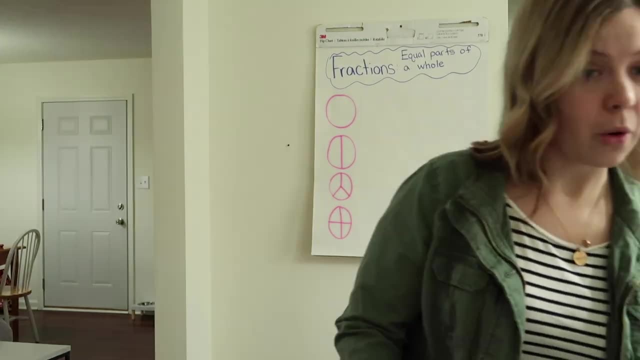 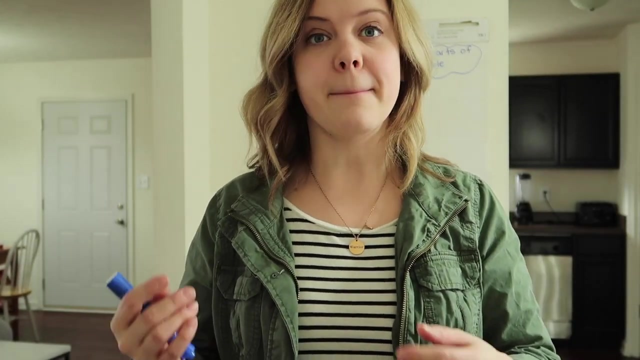 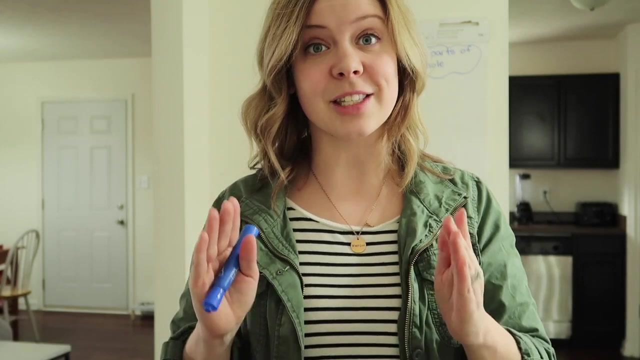 two equal halves. this is what it would look like right here: Half for you, half for me, And that's actually a fraction that we're going to talk about right now. So remember the word equal means the same. So when we're dividing our circles or squares or whatever we're dividing, make sure that equal means the same, so that all the pieces are the same size. That's very important to fractions. Now let's go up here. First of all, we've got something called 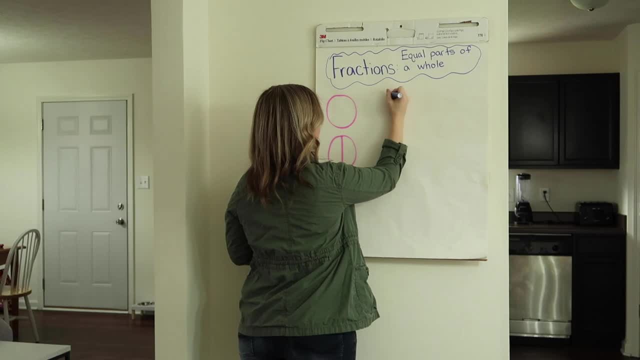 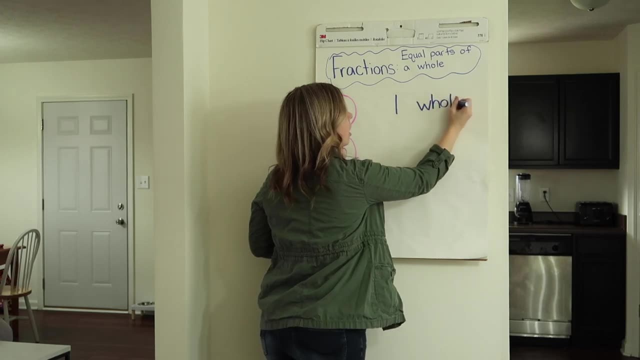 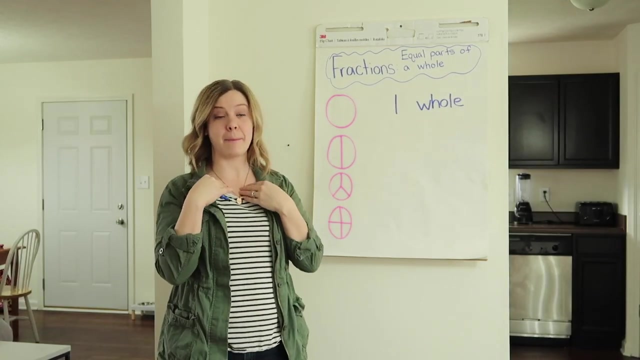 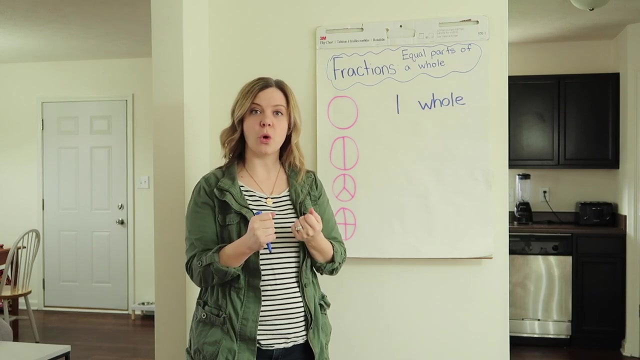 a whole. A whole looks like just one. It's one of something. We call that a whole. Can you say whole, Whole? It's one big piece. I'm not starting with anyone, I get the whole thing myself. Now we're going to talk about when we divide something in two. When we divide something in two, we call that half. Now half is represented with a fraction. 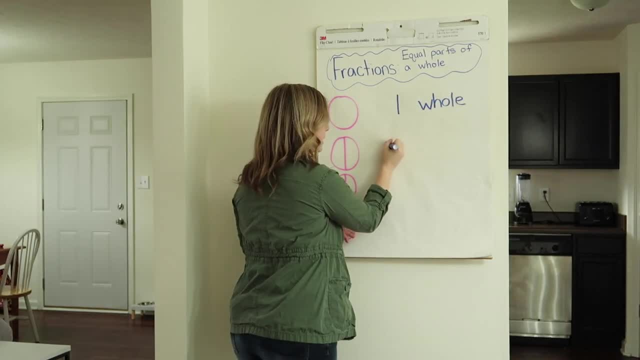 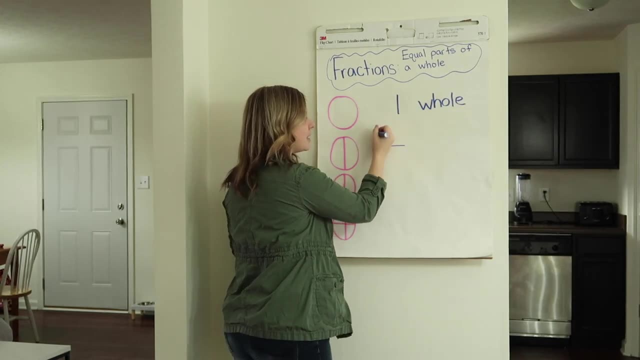 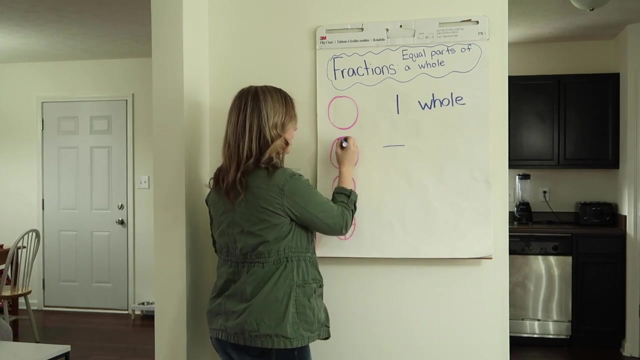 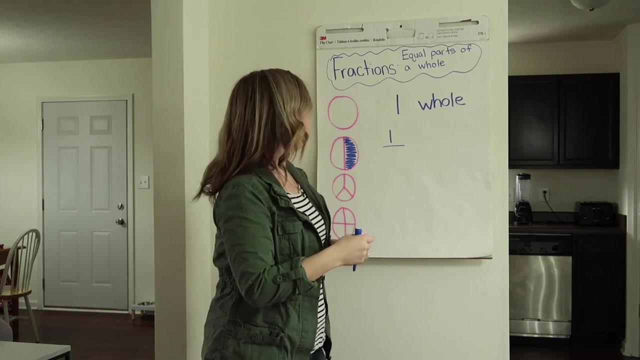 Now, with a fraction, we have this line. here We have something called the denominator and the numerator. So up here is how many pieces are shaded in. So if I had half of this in the blue, it's one, And then the bottom is how many pieces are all together. So there's one, two pieces. 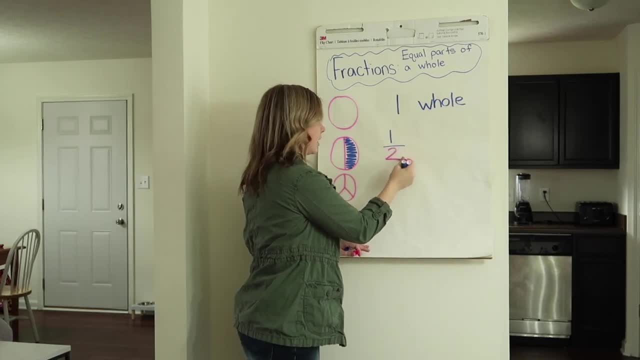 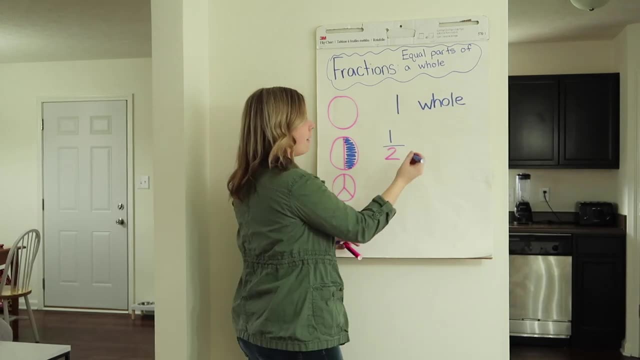 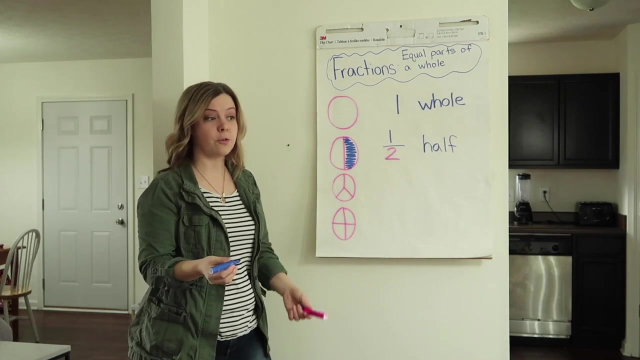 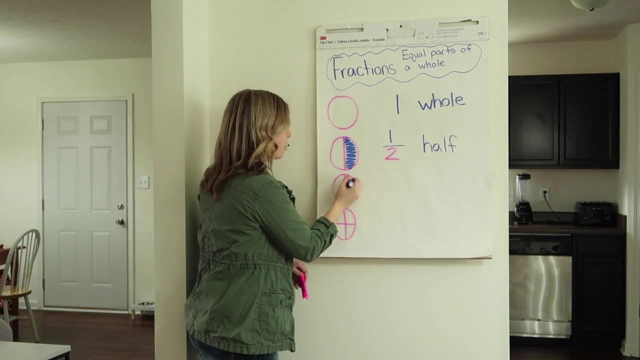 At the bottom. So it's two on the bottom. One line two is the fraction for half. So if you ever see this symbol here, this symbol is for half. Now let's move on to if we want to divide something into three pieces. Three pieces So we have three friends and we want to share this between three friends. So the number at the top is: 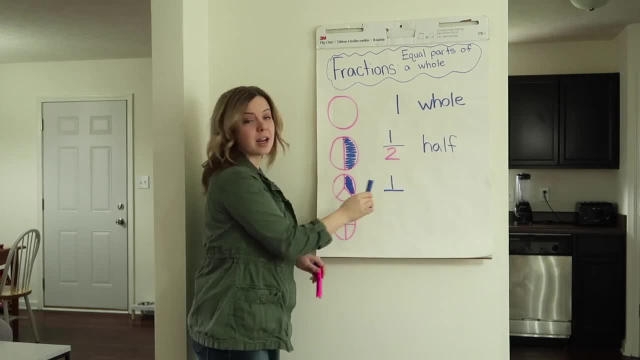 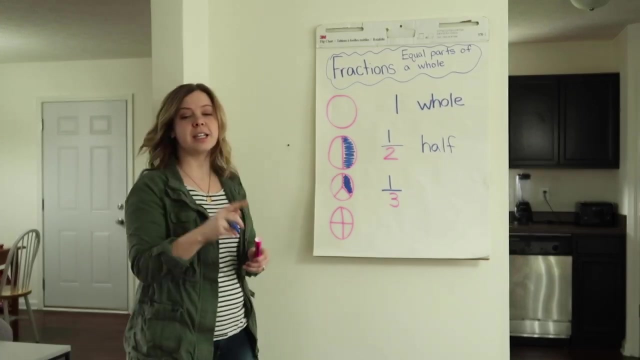 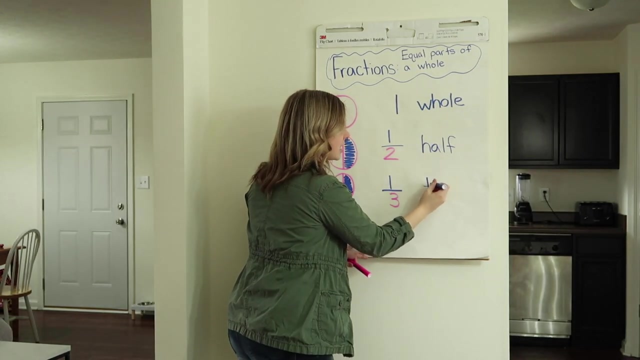 going to be one. I would do that line. But the number at the bottom is what's different? because there are not two pieces anymore, There are three: One, two, three pieces, including the shaded one. So the bottom number is three. And this is how we say: one third, One third. So we go one half, We got one third. Now, that's easy to remember, because third sounds like three and there are three pieces.